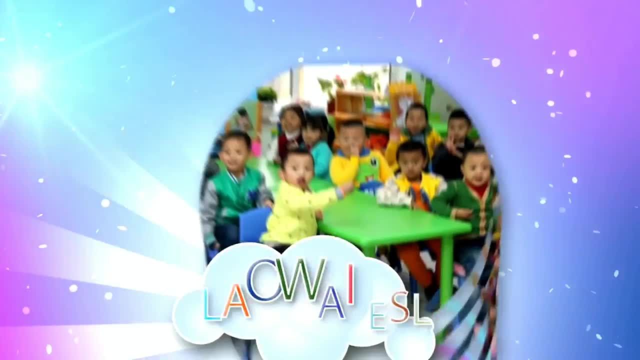 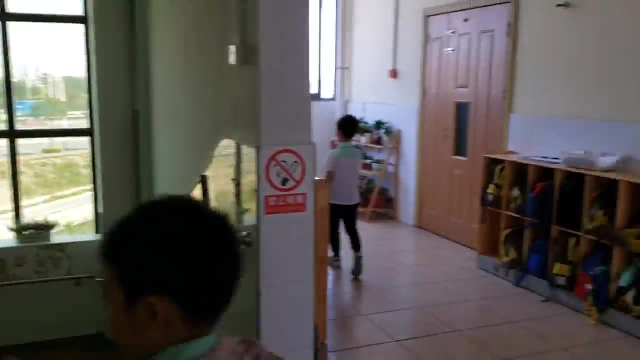 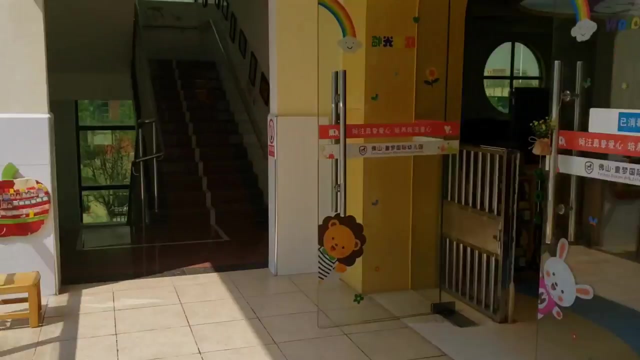 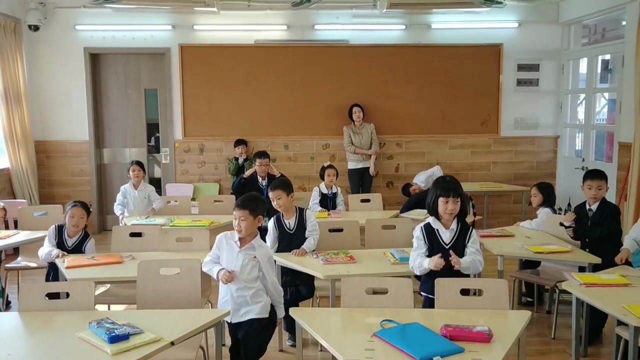 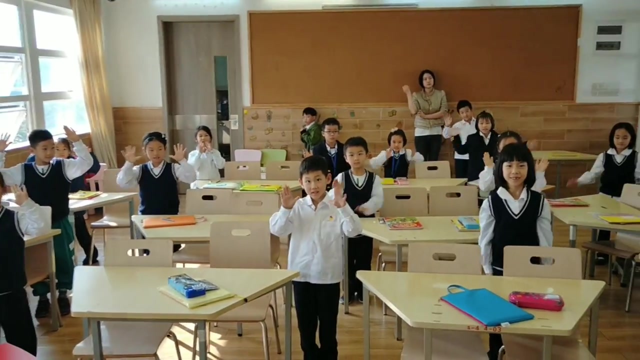 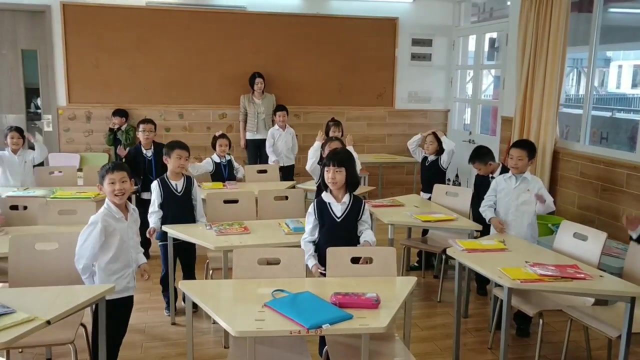 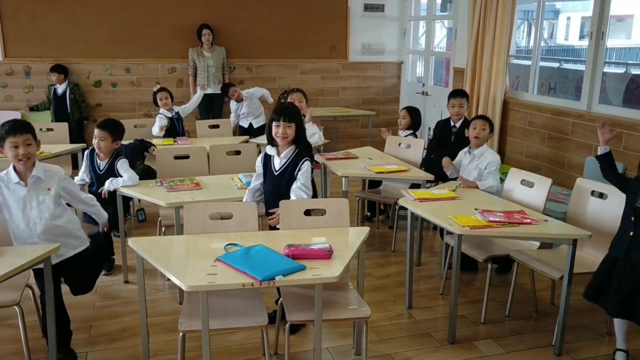 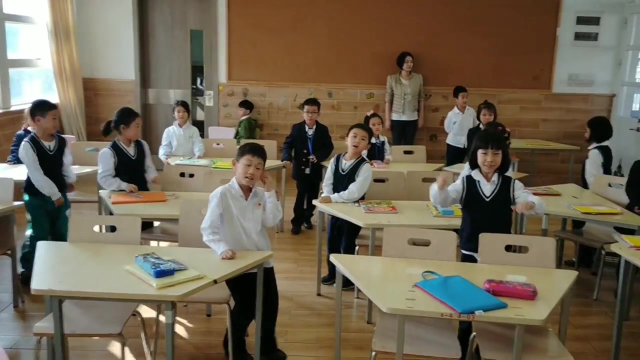 Sit down, stand up, everybody turn around. put your hands up, hands down, hands up, hands down. sit down, stand up, touch your head, touch your toes. toes clap your hands, touch your nose. sit down, stand up. everybody turn around. hands up, hands down. 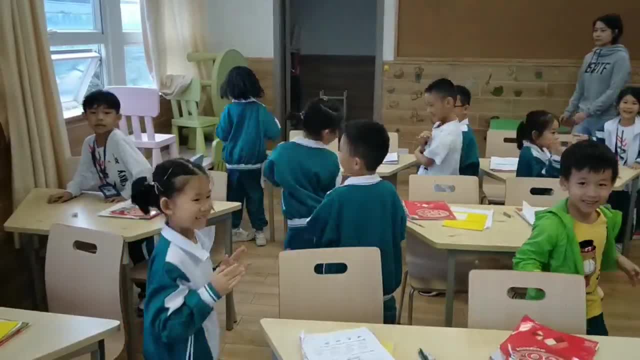 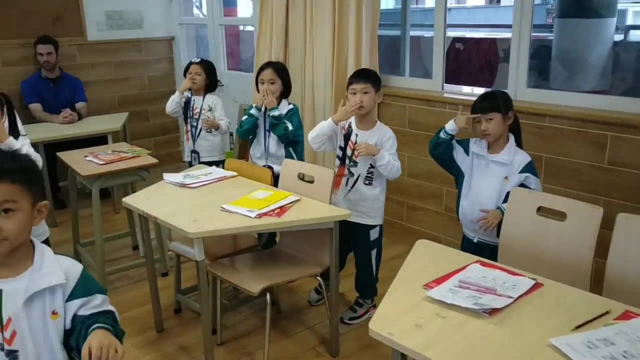 Sit down, stand up, everybody turn around, put your hands up. Let's go faster. Are you ready? Let's go, Let's go faster. Touch your head, touch your nose, clap your hands, touch your toes. sit down, stand up, everybody turn around, hands up, hands down. 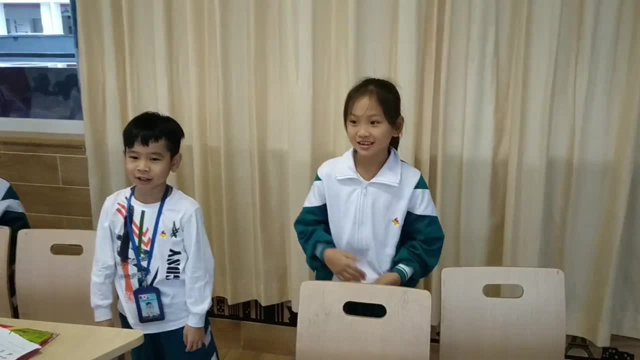 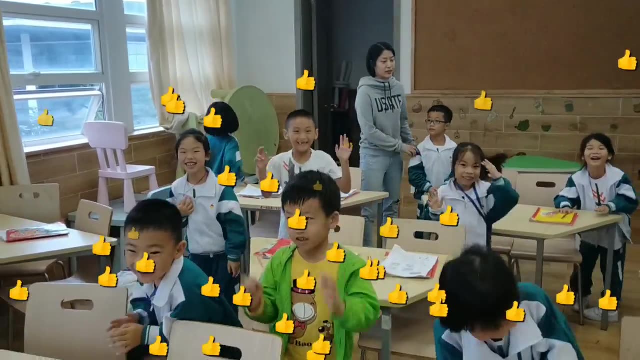 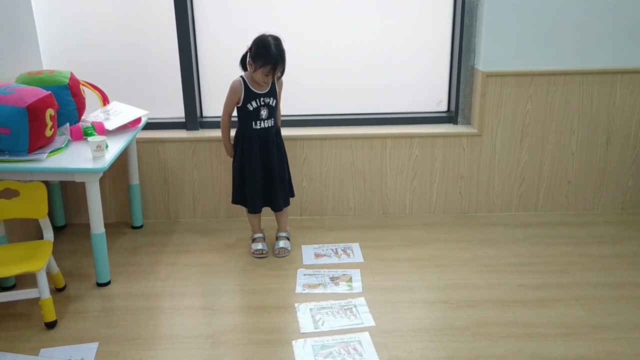 One more time. Come on One more time. Touch your head, touch your nose, clap your hands, touch your toes, sit down, stand up, hands up, hands down. Well done, guys, I can't, I'm a girl. 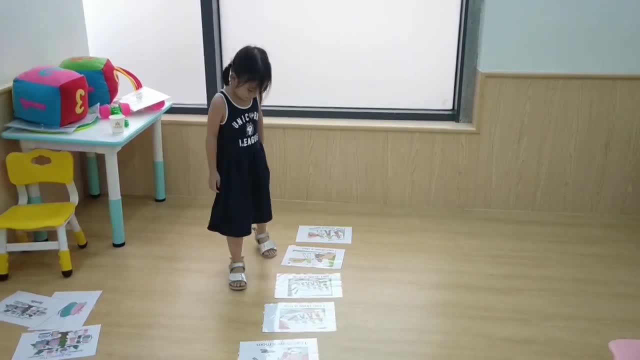 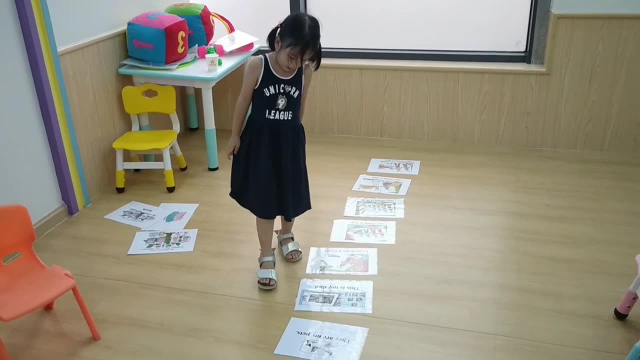 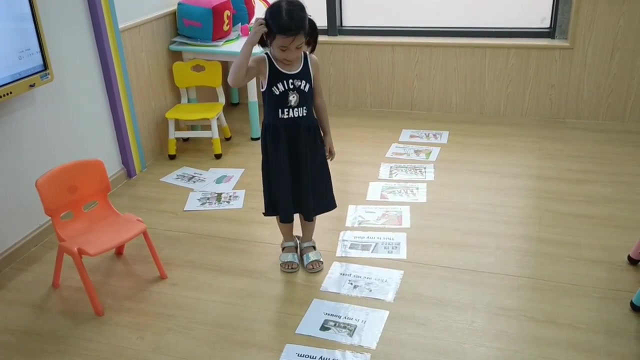 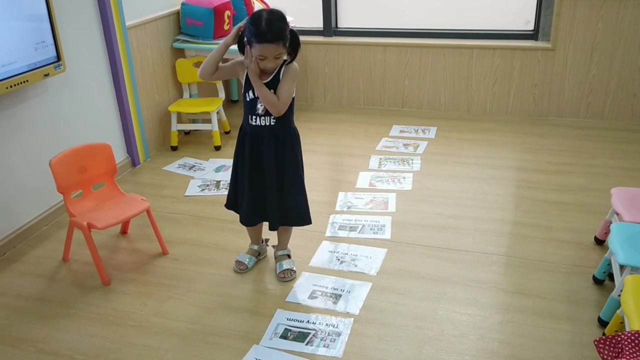 All right, I can drive a dad- Good job. I can drive a dog- Wonderful. I can drive a boy. I can drive a mom. This is my dad- Excellent. Lay on my pants- Wonderful. This is my house. 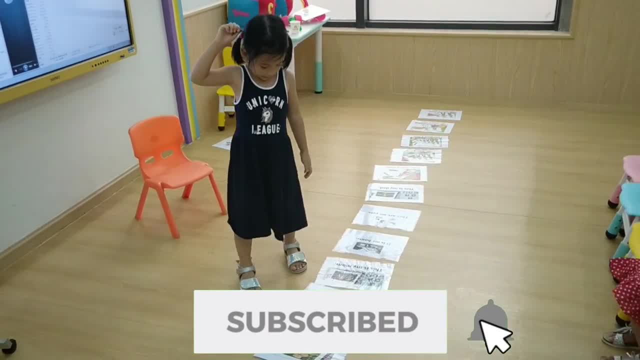 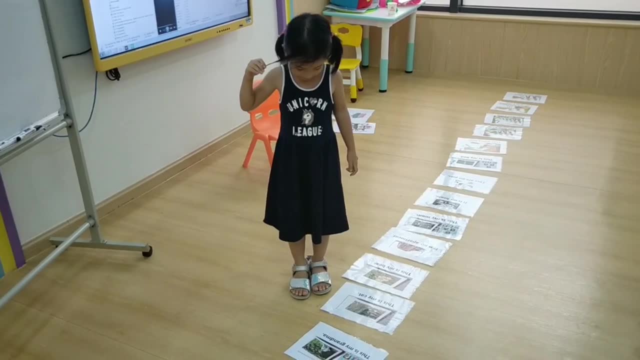 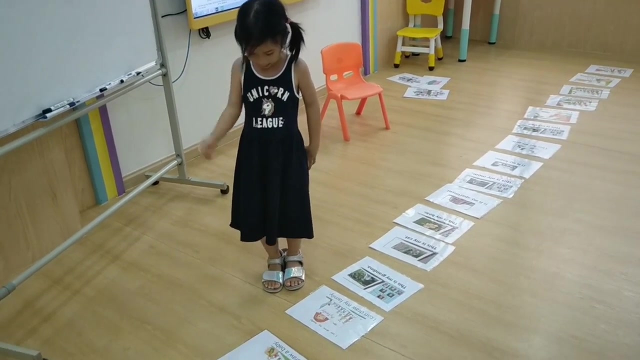 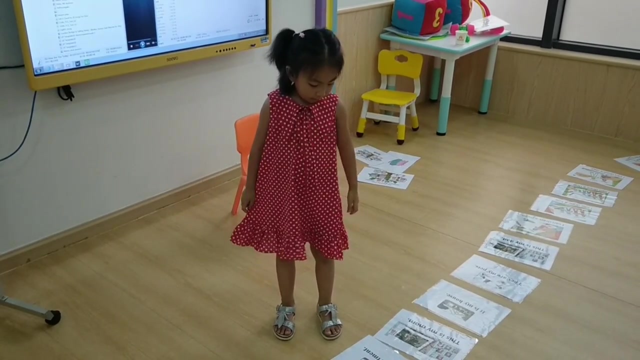 Good job, This is my mom. This is my apartment. This is my bear. This is my cat. This is my grandma. I can drive family. I can drive baby. Well done, This is my apartment. Wonderful, This is my house. 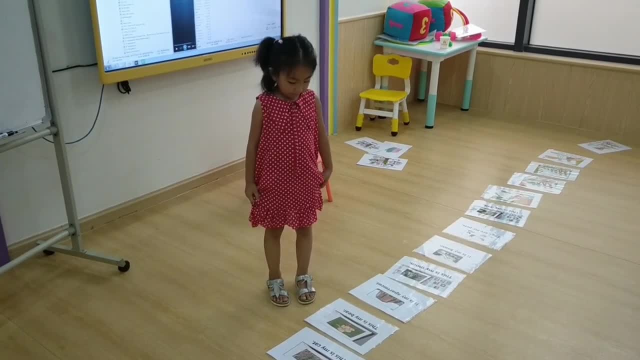 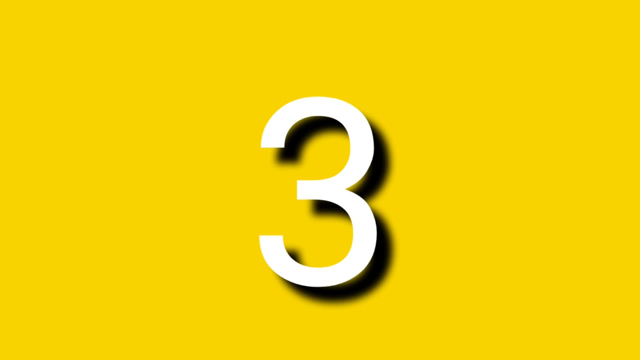 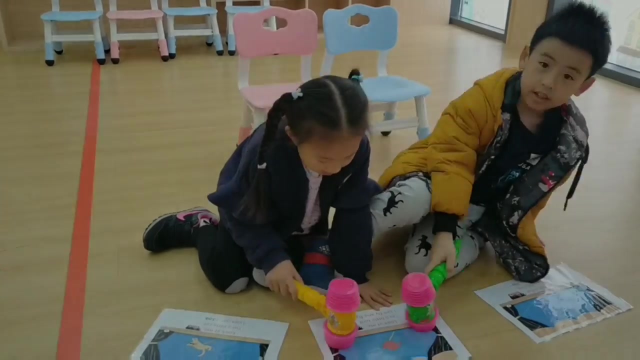 This is my apartment. This is my apartment. This is my apartment. This is my handbag. This is my ball. This is my bag. This is my bag, This is my bag. This is the last time I tell you I'm happy. 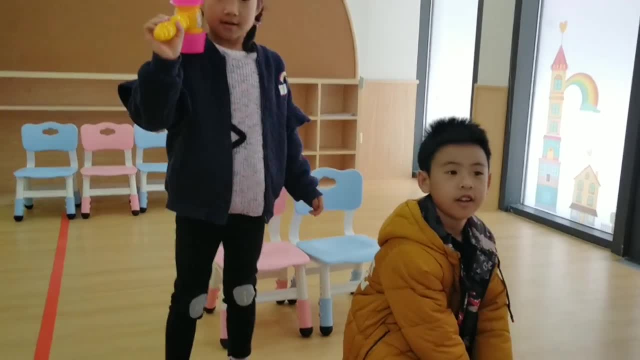 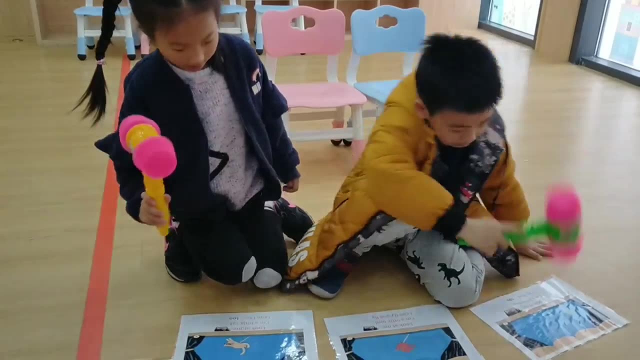 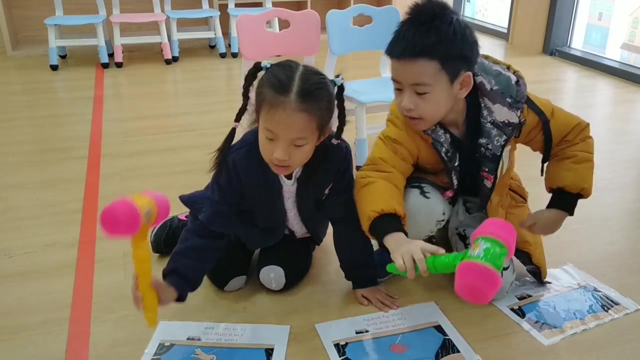 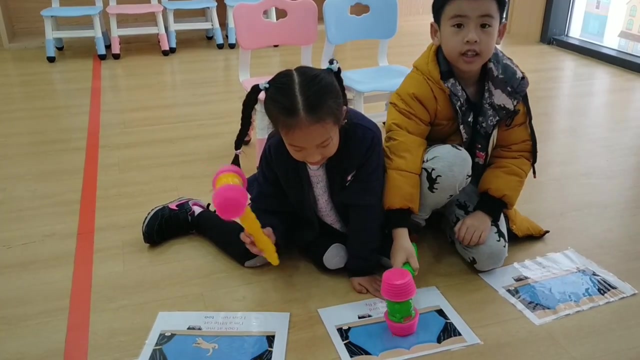 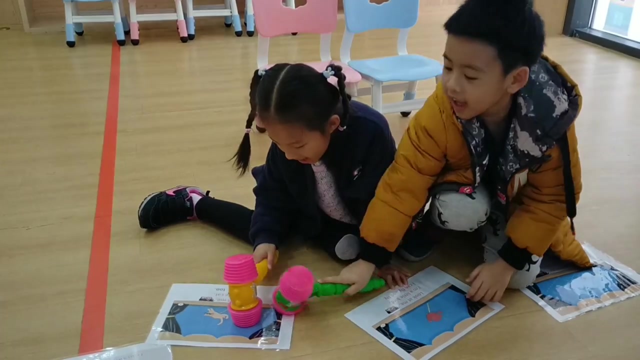 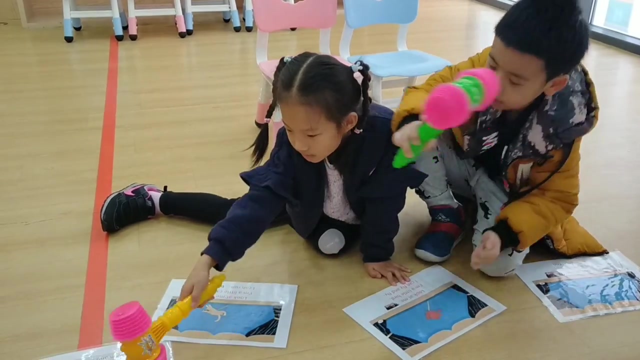 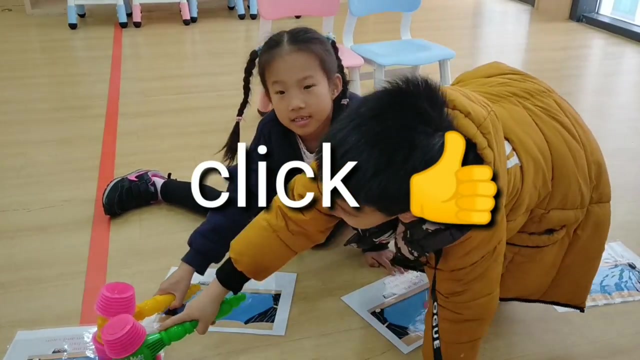 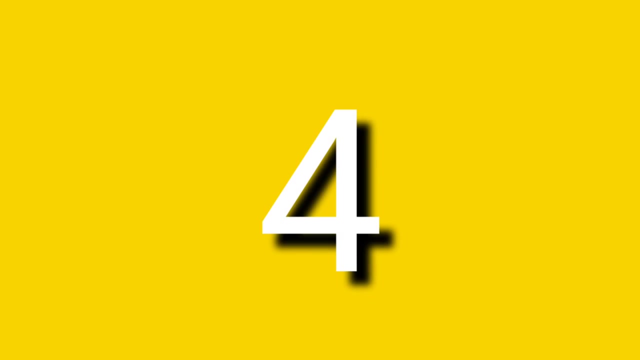 I'm happy. That's good. Good job guys. That's very good, That's cool. All right guys, Fly, Run, Swim Hop, Fly, Run, Fly, Run, Hop, Fly, Swim, Fly, Swim, Run, Hop. Angela, please find here a bag. Where is a bag? 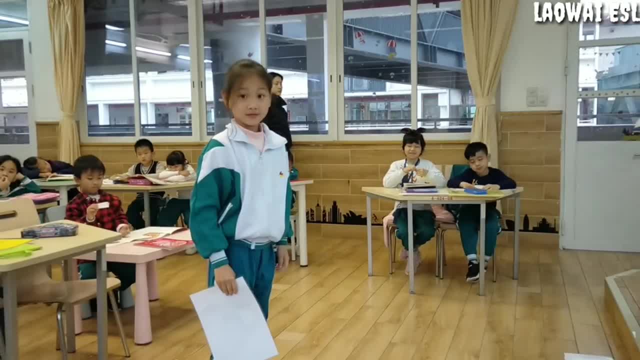 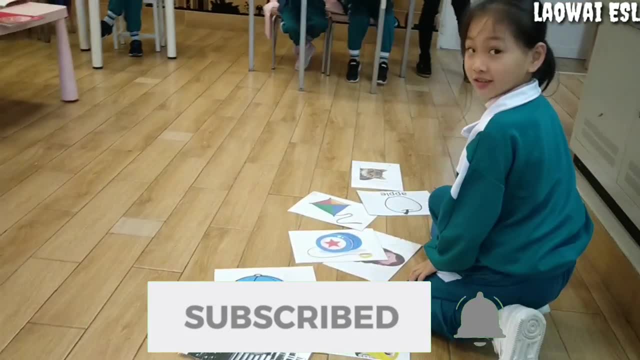 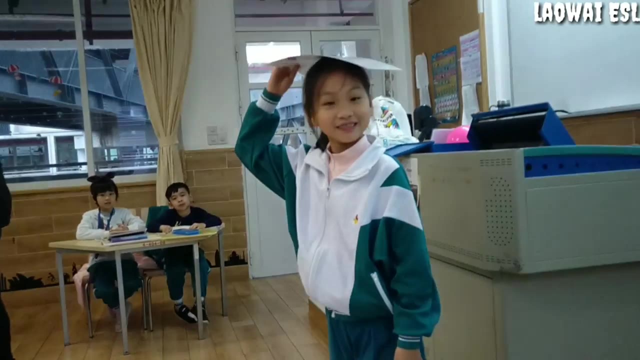 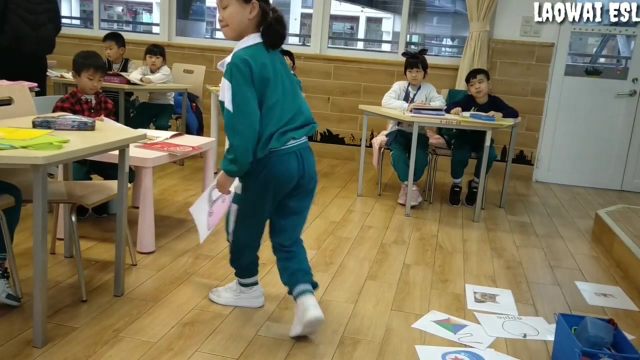 Wonderful. Now please put this bag in the box. Put this bag in the box. Okay, very good. Put this bag on your hat- Wonderful. Put it under the chair. Under the chair, Very good. Okay, come back and sit down. 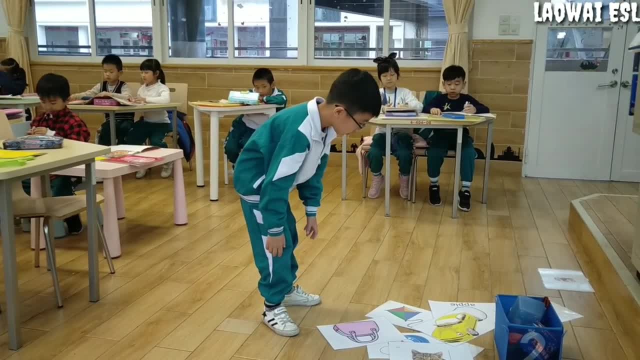 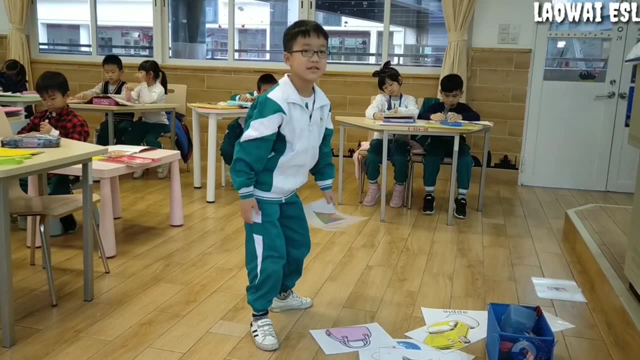 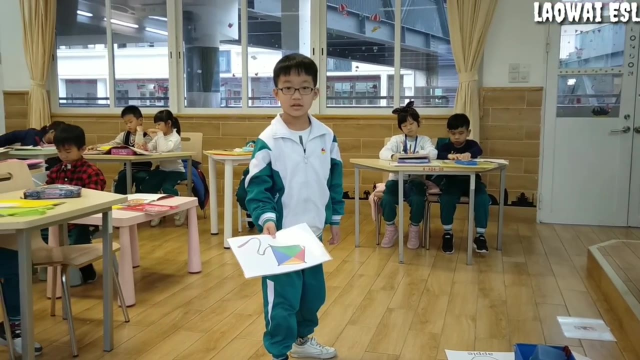 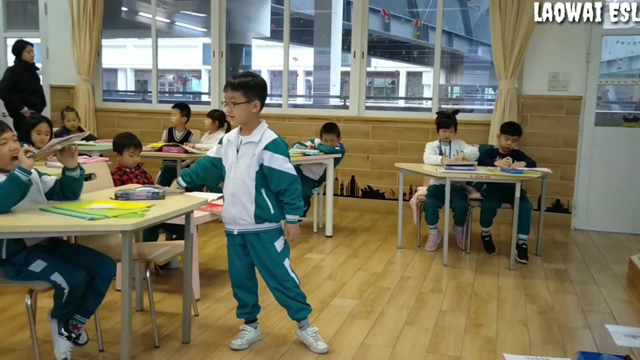 Find here a kite. Where is a kite? Where is a kite? Please put this kite on a desk, On a desk, On a desk. Very good, Now please put it on the floor. On the floor. On the floor. 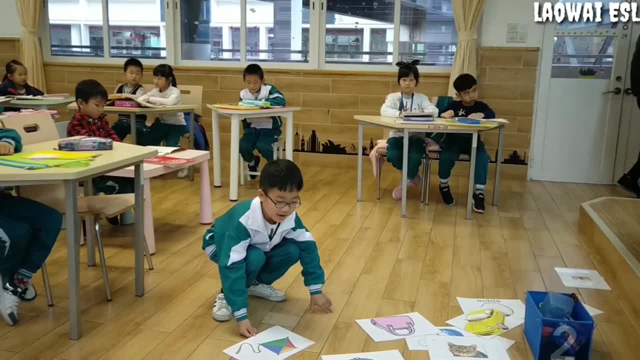 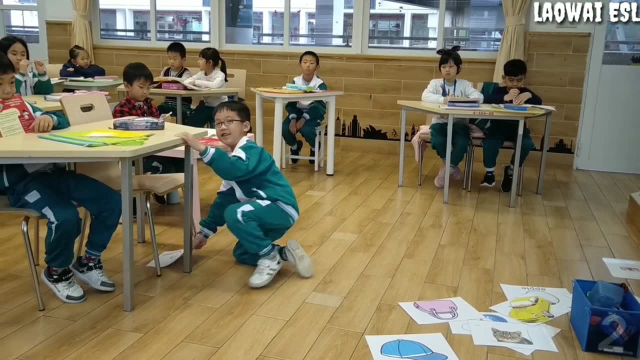 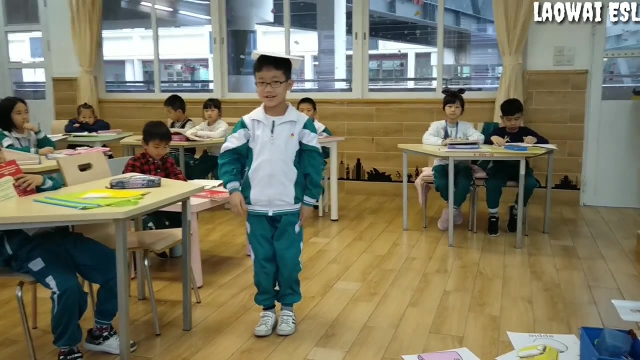 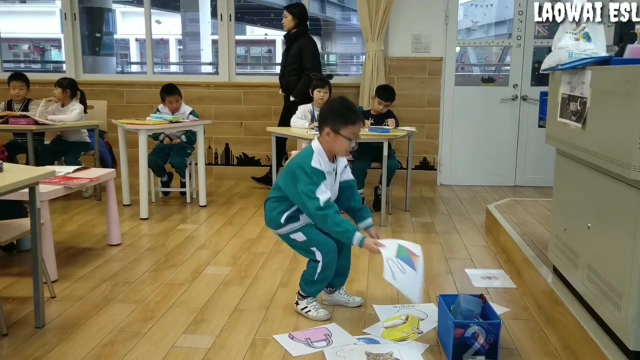 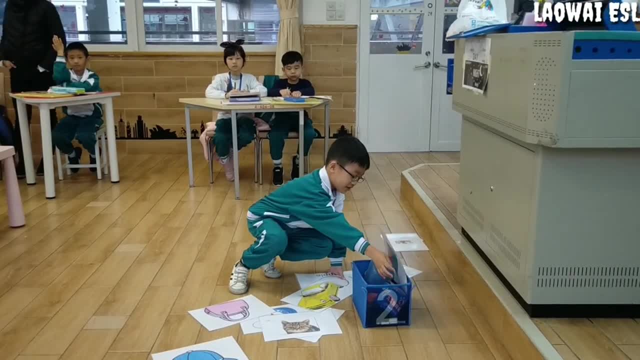 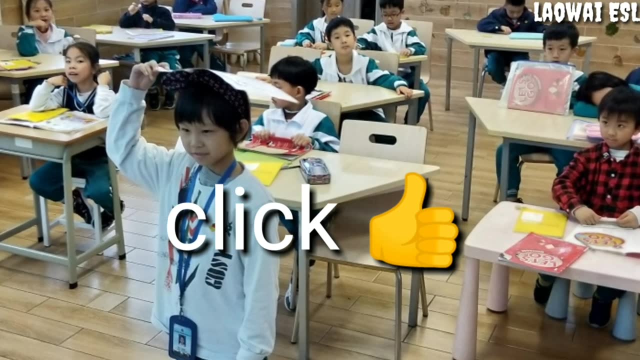 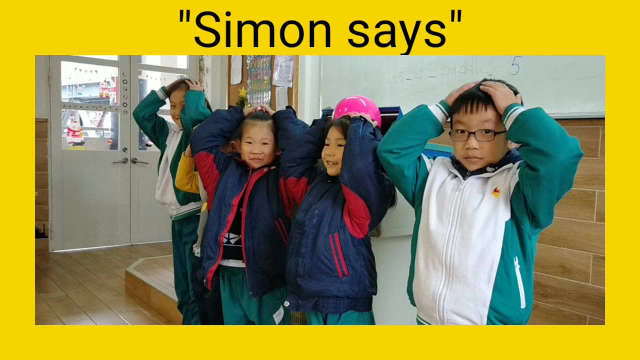 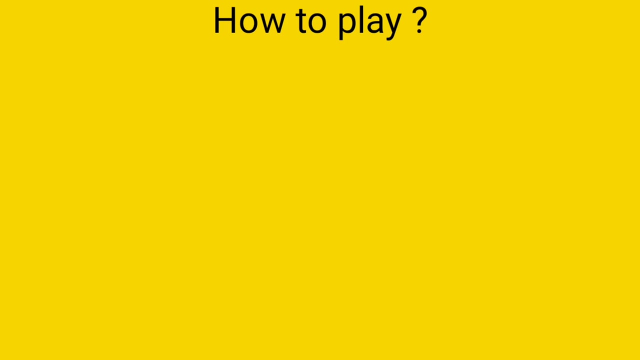 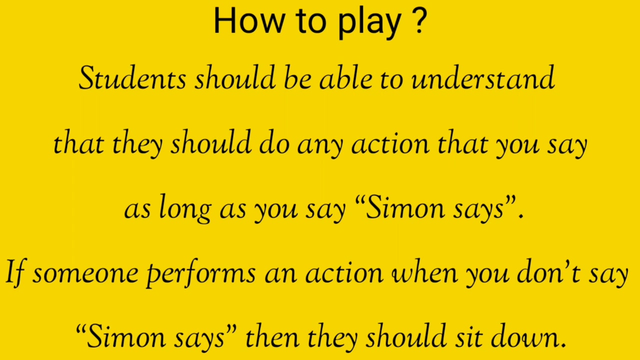 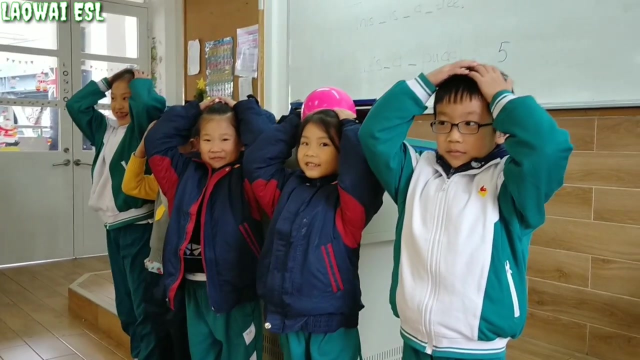 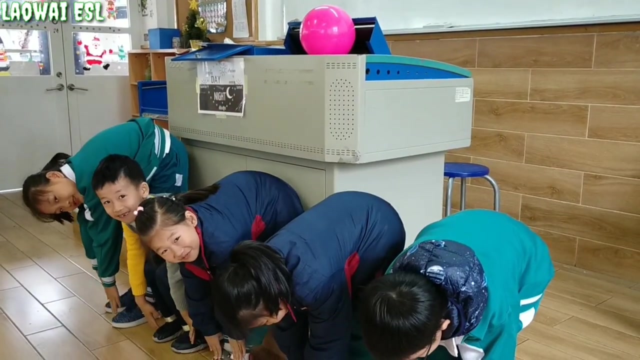 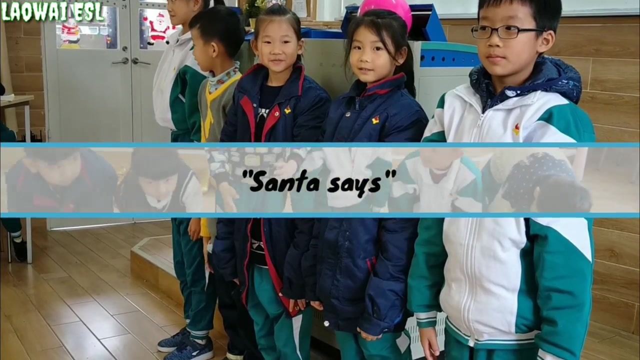 In In. Very good, Come back and sit down please. Simon says: that's your hat. Simon says: touch your nose. Simon says: touch your toes. Simon says: stand up, Sit down, Touch your hat. No, sit down please. 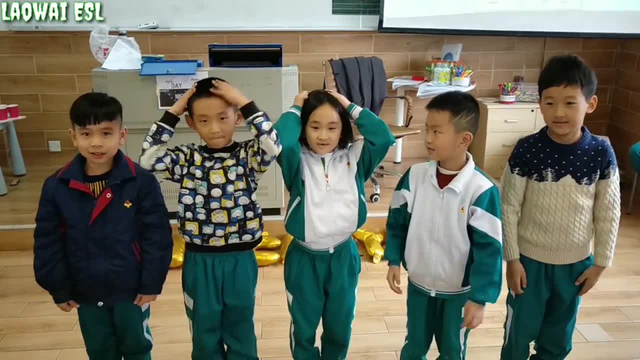 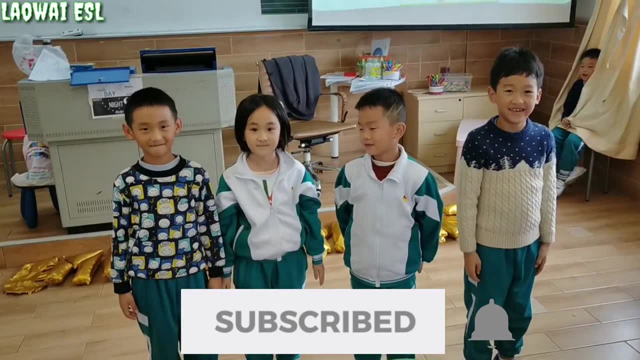 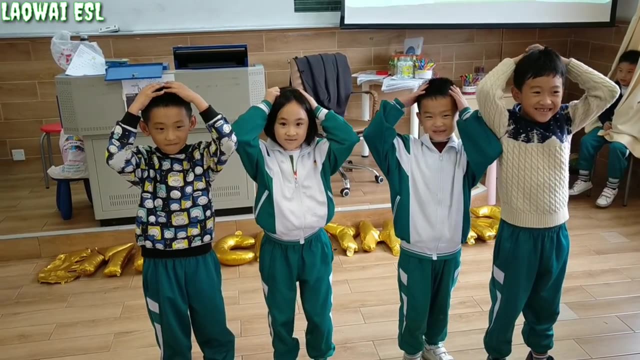 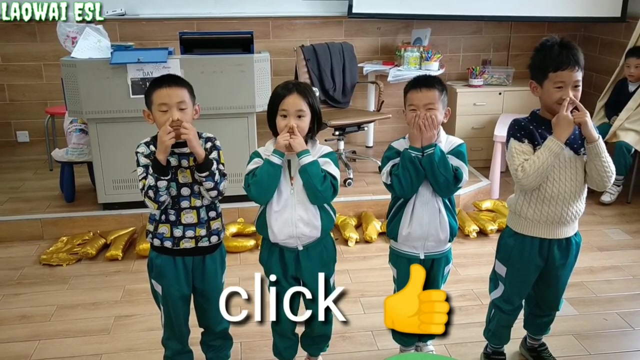 Okay, Santa says: touch your hat, Touch your nose, Sit down please. Santa says: turn around. Okay, Santa says: touch your hat. Santa says: touch your toes. Santa says: touch your nose, Touch your hat. 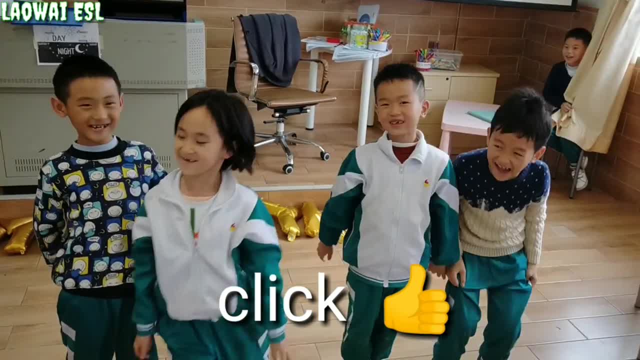 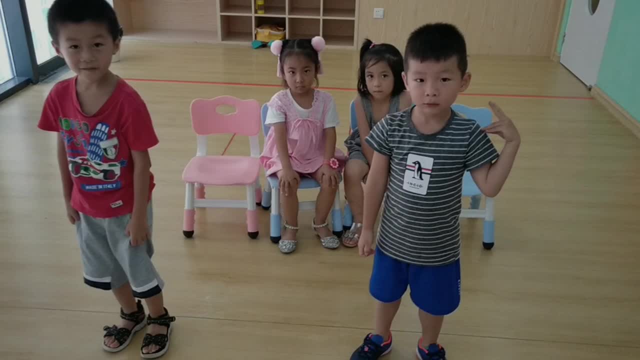 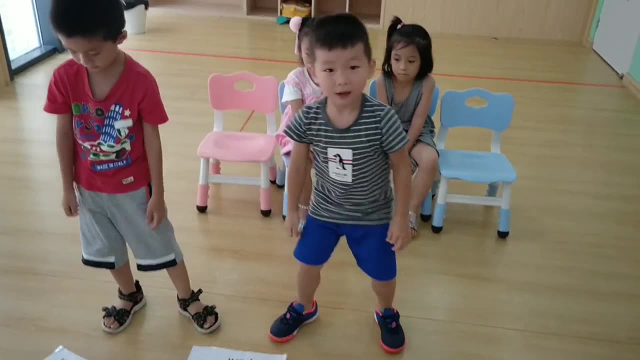 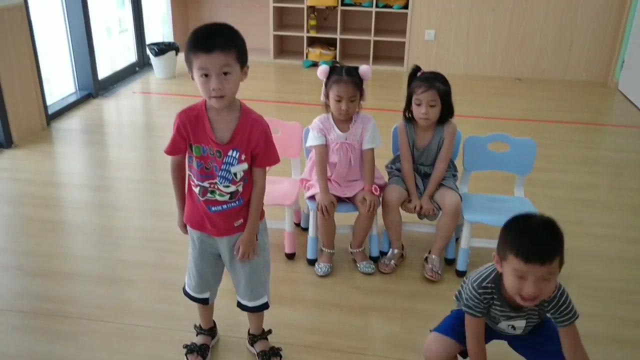 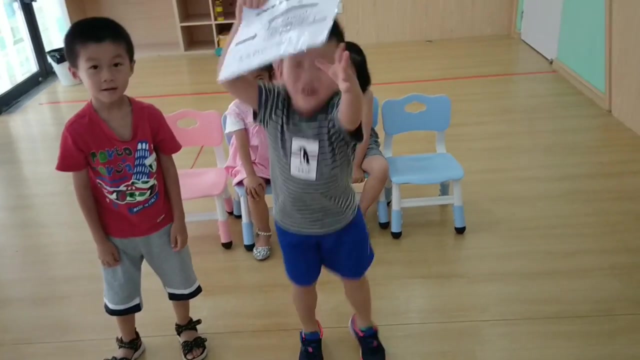 Touch your eyes. No sit down, please. No sit down, please. Three Park, No park. Very good, Police station, Police station, Good job. Hospital, Hospital, Down School, School School, Okay. 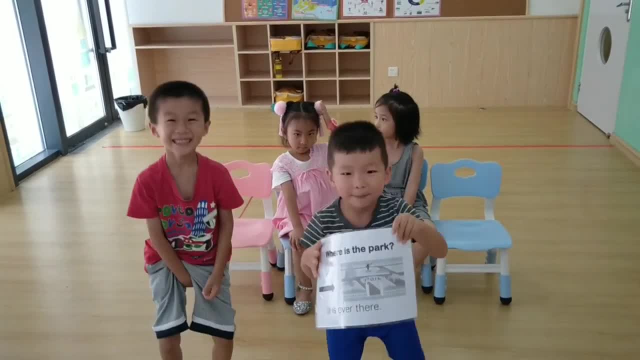 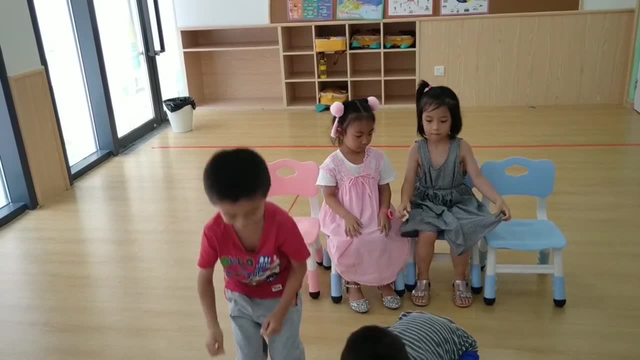 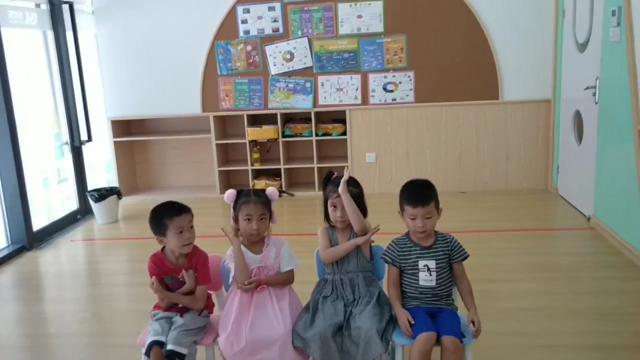 Park Park Park Park. All right, three Police station Police station: Park Park Park Park Park Park Hospital Hospital. Park Park Hospital Hospital. If you want to play, please raise your hands. 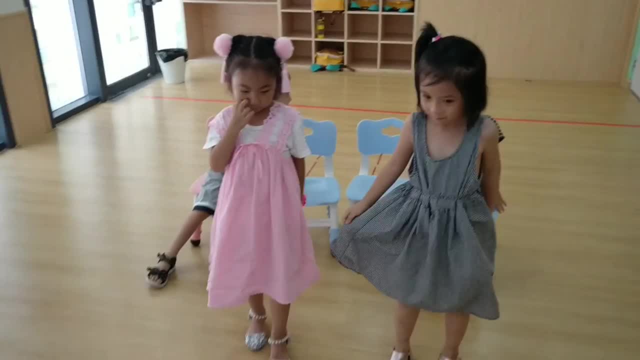 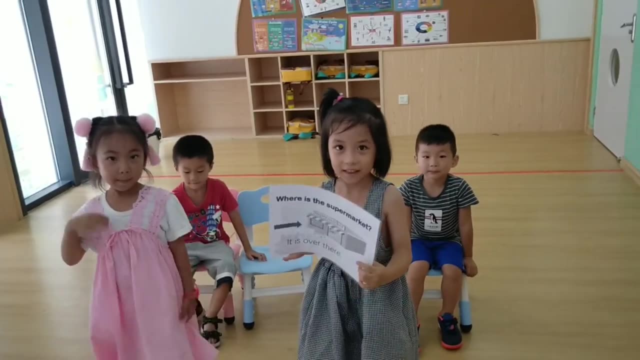 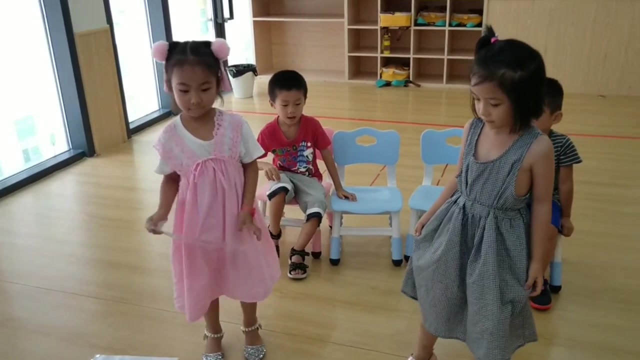 Okay, stand up and come here, Tell me, are you ready? Yes, One, two, three Supermarket, Supermarket, Very good, Okay, School, School, Wonderful, Wonderful Hospital, Hospital, Hospital, Okay Park. 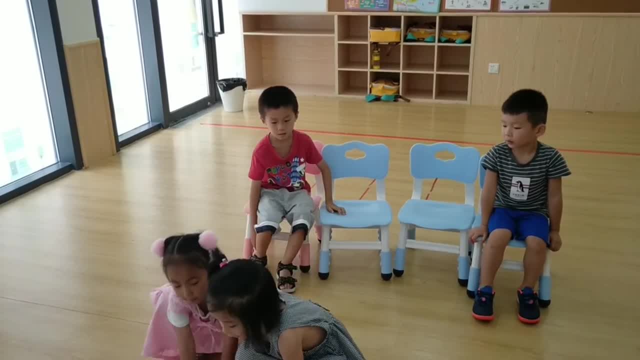 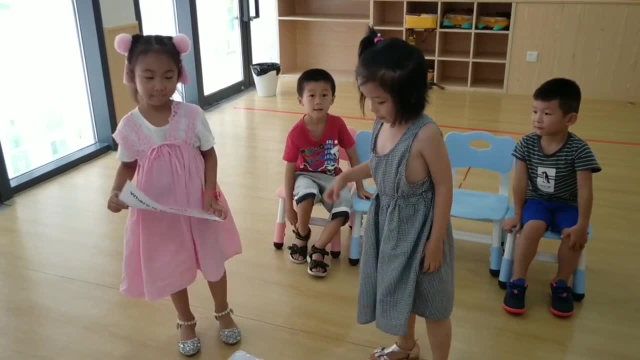 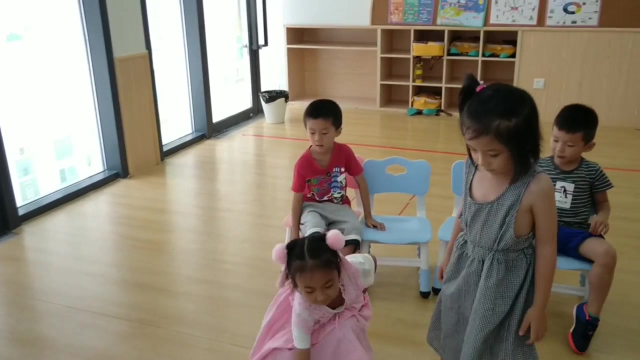 Park Park, Park Park Fire station, Fire station. It is a police station, A police station, A police station. Very good, Supermarket, Supermarket, Supermarket. How Supermarket. Wonderful School, School.